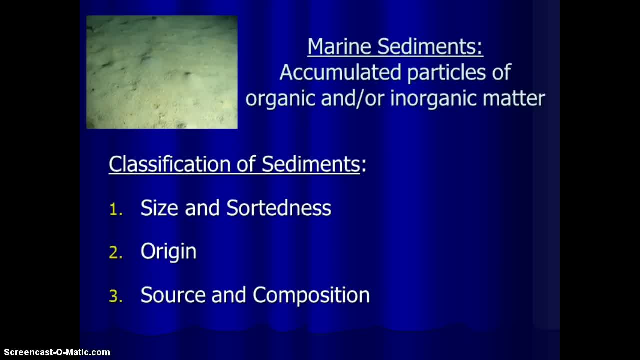 And these will be something that comes more into play as we do primary production and as we actually talk about the benthic environment in terms of ecology and biogeochemical cycling. But for this lecture, we're going to really quickly just go over the different types of marine sediments, where they come from and which ones are most prevalent, And essentially- as it will be with the rest of the course- we're going to start with basically defining the sediments. So how do we define them and classify them? 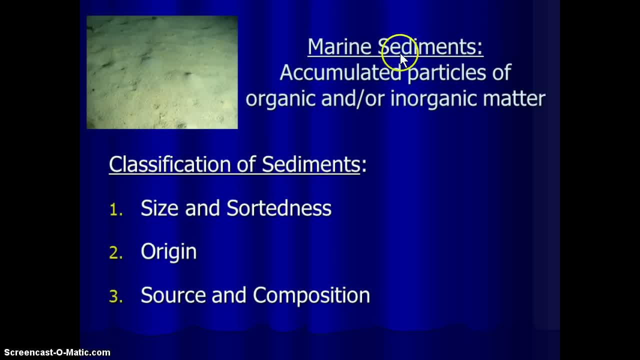 So the definition of marine sediments really, or any sediments, is the accumulation of particles, whether they're organic or inorganic, and that means are they generated from a living source or a non-living source. We'll classify them in several ways. We do classify them according to size and sortedness, and I'll explain what that is only really briefly. 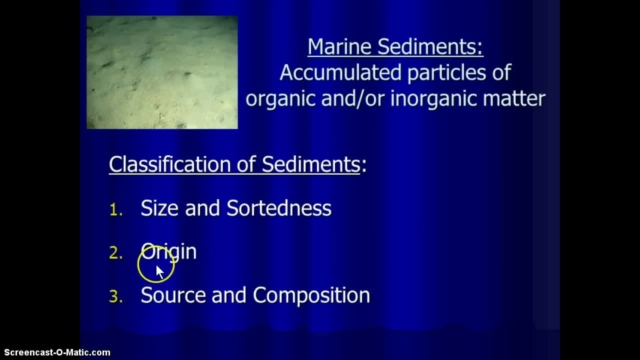 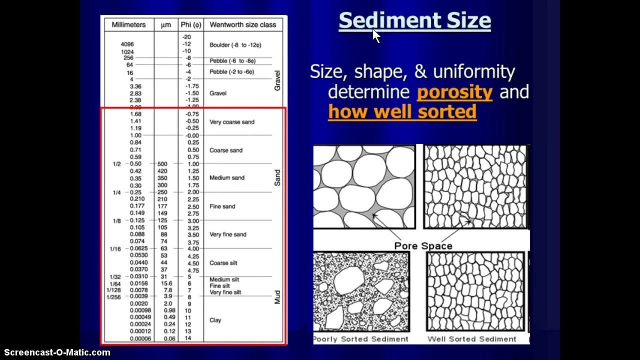 And then origins, so where they come from, or how they're formed, and source, where they come from And composition are really the two main things that I'll focus on or that I'll hold you accountable for, really. But first the sediment: size and sortedness. And size is self-explanatory, sort of how big are the particles? 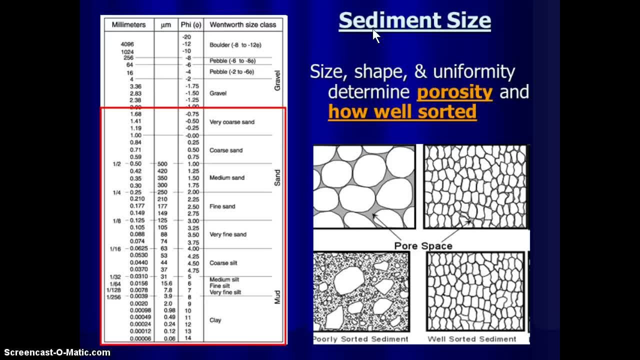 But it has a lot to do with where the sediments lie is very dependent on their size and mass, But also the size combined with the shape uniformity. So are they all pretty spherical? Are they all amorphous? They have angular and un-uniformity. 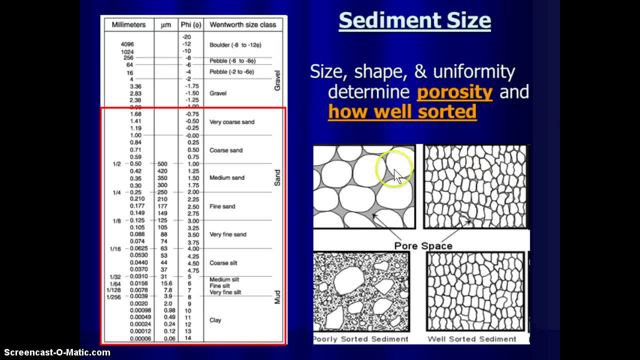 And un-uniform shapes. that determines its porosity, so how much space is in between each particle here and it also determines how well-sorted it is. Now, if we just look at size, if we look at all these things together, we can come up with a phi number, which is basically a measurement of how well-sorted they can be. 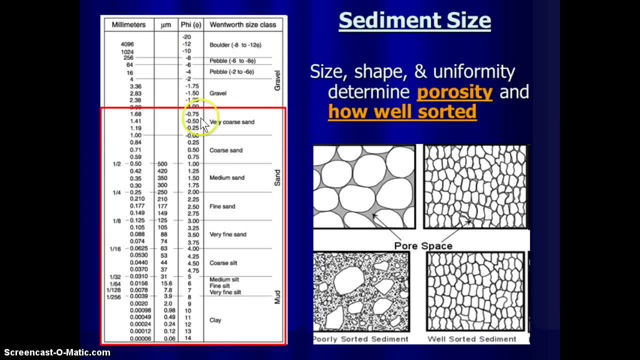 But I'm not going to hold you accountable for that at all. But what we do find is that the majority of sediments- marine sediments- are made up of you know, a wide variation in sands and silts and clays, And these are determined by their composition. They're all mineral particles, which means they're broken down, rocks and size. 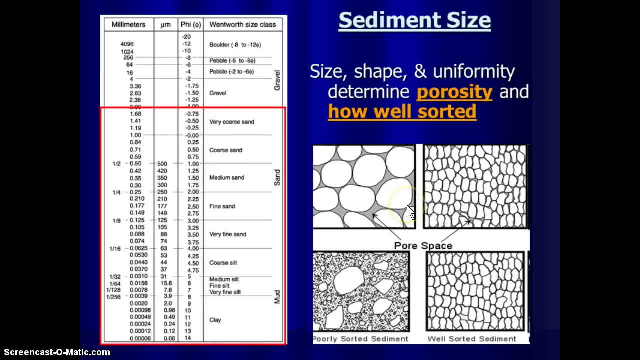 But how well-sorted they are is. so if you have, you know, very uniform versus very un-uniform sediment particles, they can either pack together very well and be very well-sorted, which usually reduces their porosity, or not be packed together very well. 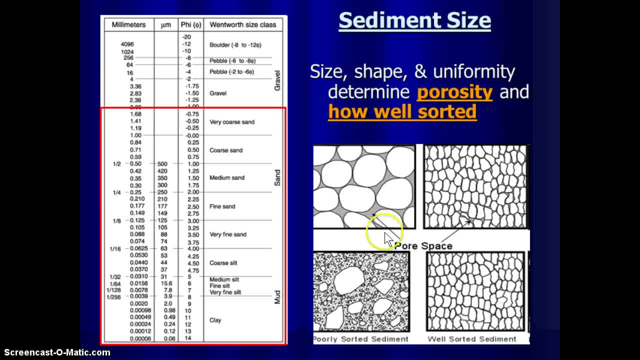 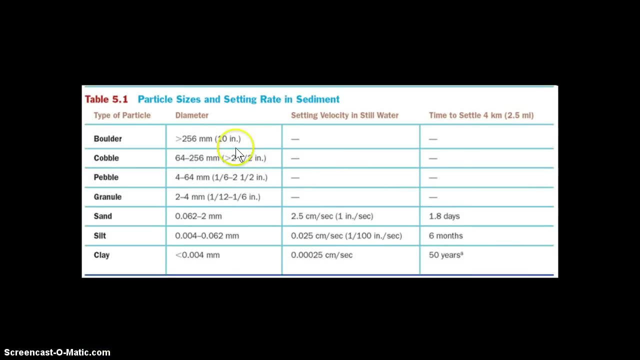 which usually increases their porosity, leaves more spaces here. And then, if there are many different types of sediments all packed together, they usually sort very tightly and leave low porosity. also, Whoops, skipped one. The other thing about size and mass of a particle determines its sinking rate. 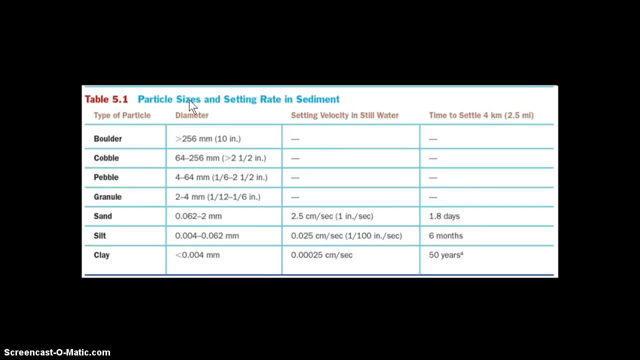 And we'll start to talk about sinking of particles over and over again throughout the course and its importance. But so the size of something definitely, and mass of something definitely has a very strong effect on how quickly it's going to sink. So, essentially, if this was settling velocity, 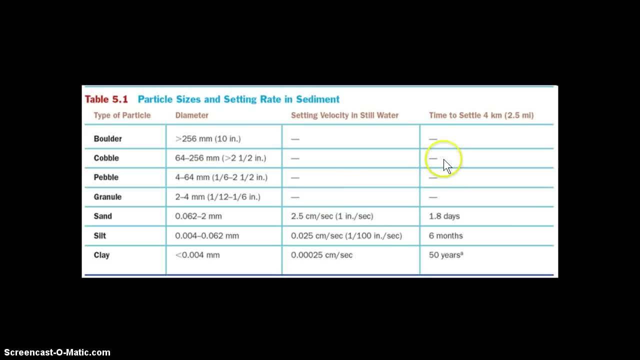 and time to settle over four kilometers of ocean, which is about two and a half miles of ocean. you know these large guys, boulders, which are ten inches or bigger. all the way down to a pebble, they really settle quite quickly. 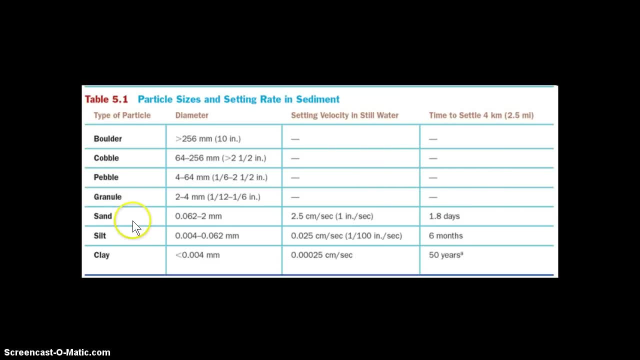 So we don't even have a number there. But when we get to sand- you know a sand that is no greater than two millimeters- they start to have pretty slow settling rate in the ocean And it could take almost two days without currents for a piece of sand to settle over 2.5 miles or four kilometers. 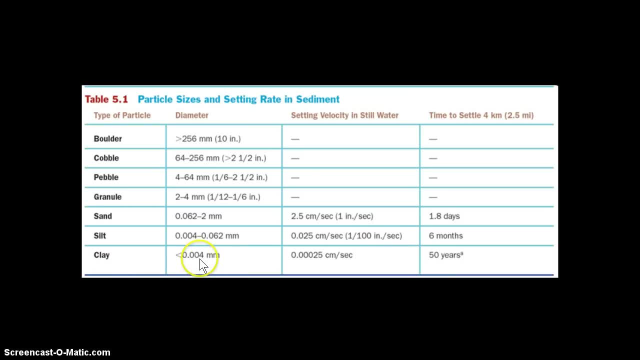 And when you get as small as a piece of clay which is .004 millimeters large wide, you get a very slow settling rate And it can take up to 50 years for that piece of clay to settle from the surface over four kilometers of ocean. 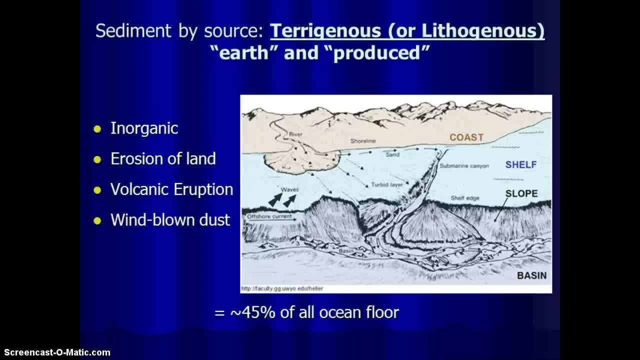 So that gets to become very significant. Alright, let's move on to source and origin. So the first source of marine sediments is what we call teriginous. It's also called lithogenous, But if we break down genus, I always find breaking down the terms. 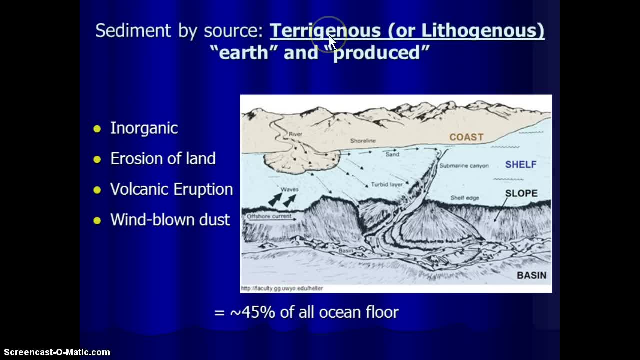 and I'll do this over and over throughout the course. break down the terms into their meanings or try to remember it in parts and you'll remember what it means. So teri means earth, teriginous terra, And genus means produced. 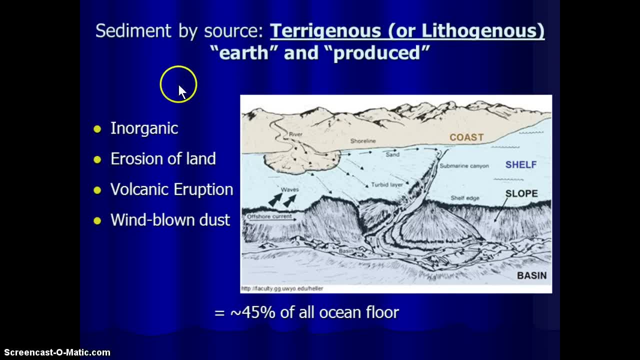 So what these mean is they're produced from earth. So teriginous sediments are inorganic because they come from the erosion: Erosion of land- essentially Rock that has formed prehistorically gets broken down through erosion and is washed through the water cycle into the ocean or onto the beach. 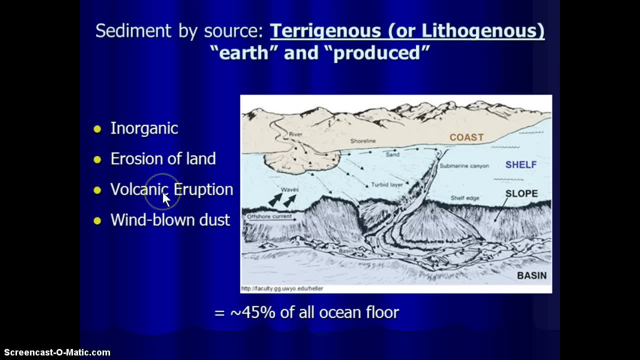 and settles and becomes the sediment. A similar thing happens from volcanic eruption: It will disperse many mineral particles into the air and settle, And then also sands and dirt on land which come from the same sources: erosion of land, volcanic eruption. 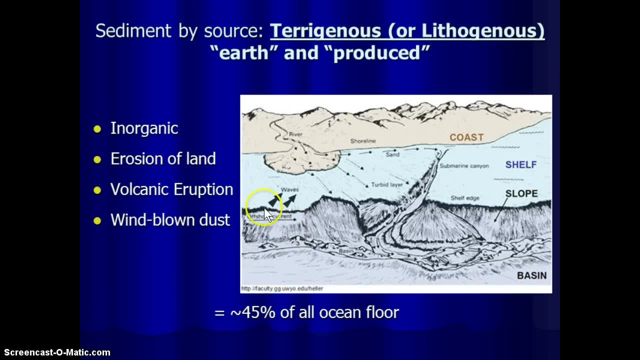 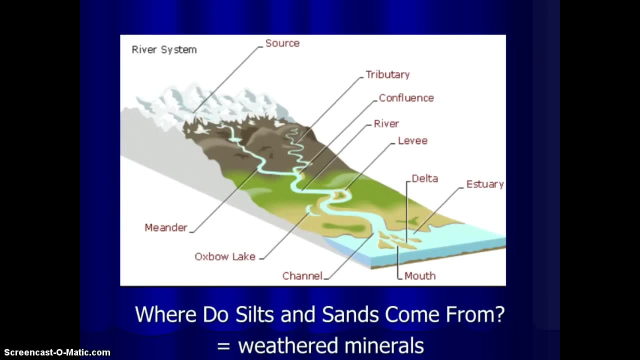 can get blown with storms into the ocean and eventually settle and become a marine sediment. And this is a very large portion of all marine sediments across the globe- roughly 45%. So that's quite a big percentage. So where do the silts in the sands come from? 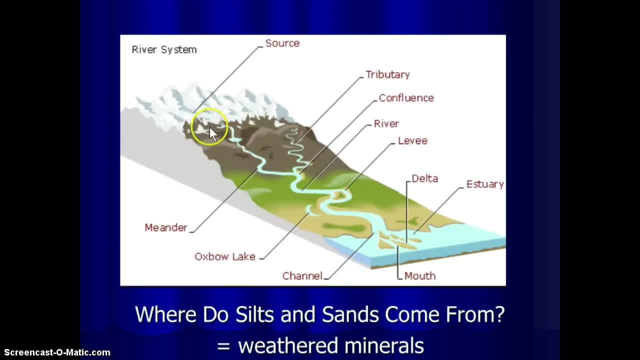 Well, we spoke of that. They start out as rock and then they're either eroded by wind or water or glacier movements. They end up washing into- you know part of the water cycle- tributaries of rivers, rivers washed down and then either settle on the coast or in the ocean. 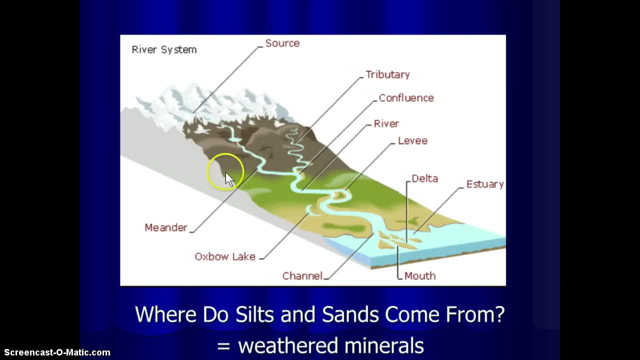 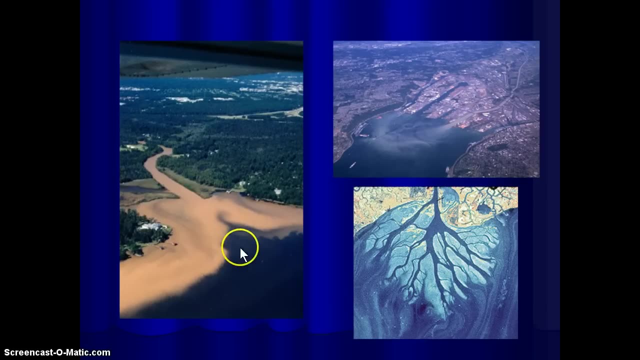 or they can be actually picked up by weather, by atmospheric circulation, and blown in on the wind and into the ocean. So essentially we're talking about weathered minerals, pterygianus. We see them wash down river deltas and settle out into the ocean. 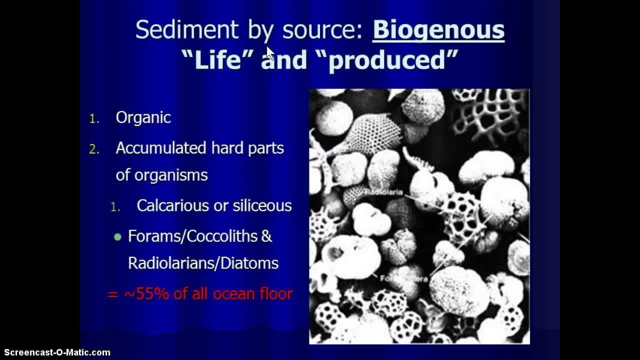 So the next and the largest source of marine sediments is what we call biogenous, or biogenus, So we can break that down, biology, and produced, So produced from life. Okay, so these are obviously from organic living sources And essentially they're the accumulated hard parts. 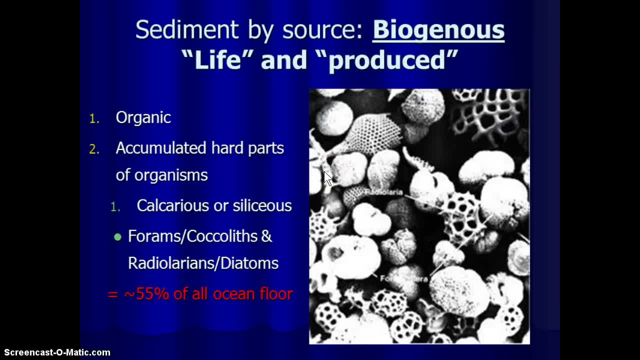 or the shells or any other hard part of an organism after it has died. Many of the organisms in the ocean, especially the microscopic ones, organisms such as forams, coccoliths, coccolithophores, I should say radiolarians. 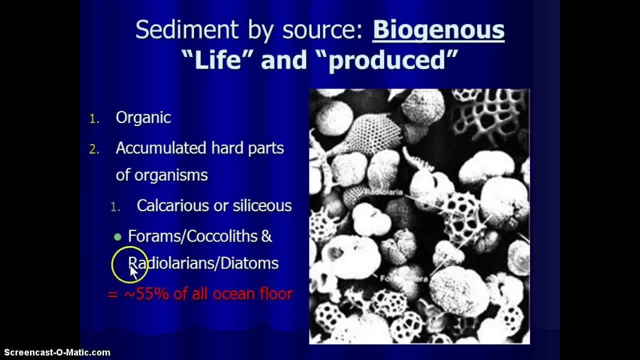 diatoms and we're going to go over these guys in much more detail in our primary production and heterotrophic lectures. But these guys form shells, You know. whether it's out of calcium or silicon or some combination of the two, they form these shells that are heavy when they die. 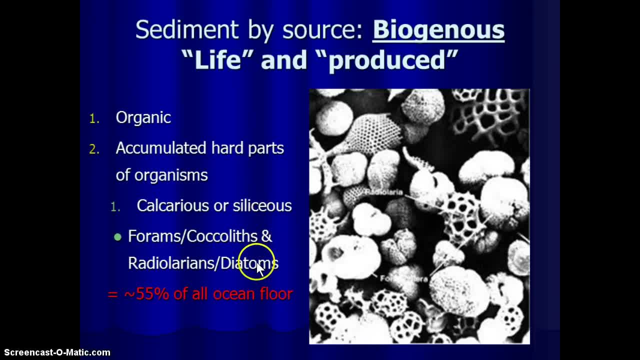 or heavy enough to settle. Anyway, when they die they settle down to the ocean floor And these make up 55% of all the ocean floor. So I said around 55 for biogenous and around 45 for lithogenous, which basically makes up 100%. 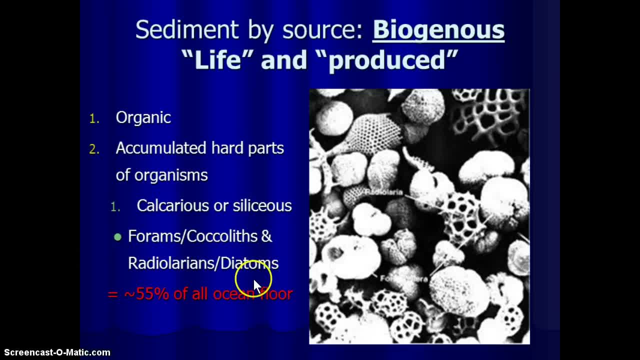 But it's really a little less than 55,, a little less than 45. And so there's this very, very small, less than 1% that makes up the rest of the sediments, But biogenous, so most of the marine sediments come from an organic. 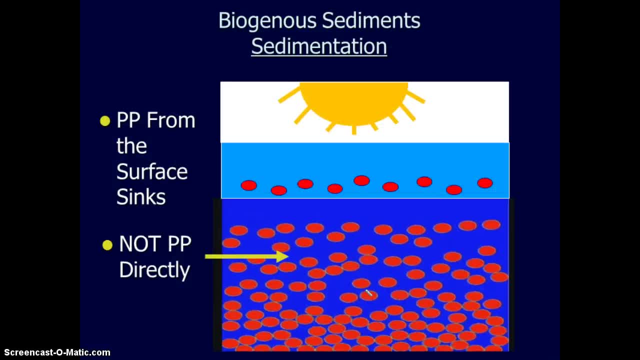 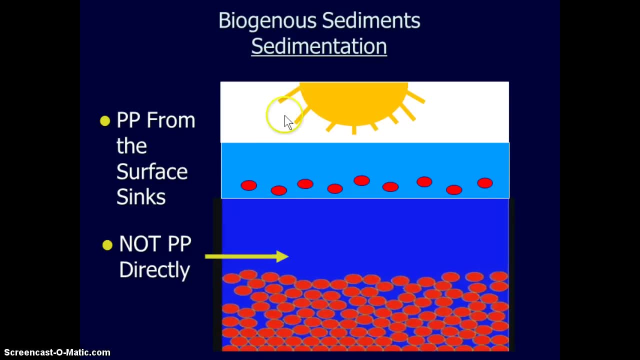 originally from an organic source. How does that work? Biogenous sediments form through. well. sedimentation Seems kind of obvious. The process of sedimentation is life grows in the surface ocean, just like plants do, and eat just like other organisms do. 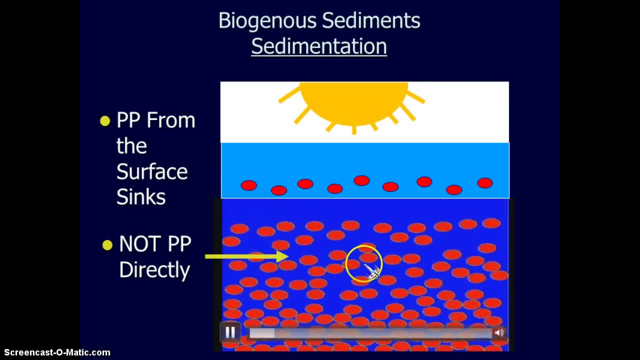 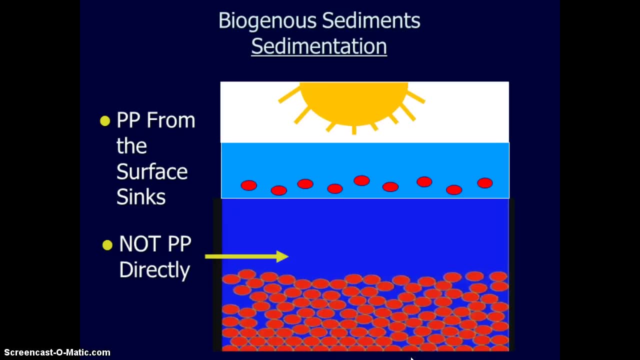 And when they die, they settle out through the water column, just like we see here, And when they settle off into the bottom, they form the sediments- PP standing for primary production- And that's really the main source of the organisms that settle. 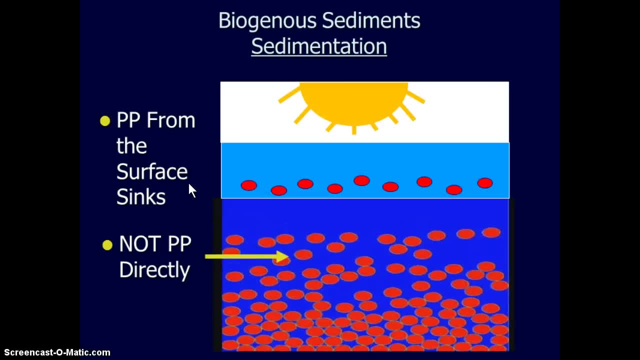 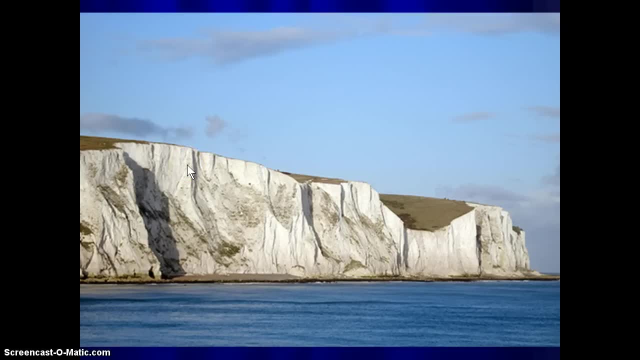 but not just primary production, And we'll talk about that some more in a later lecture. Some of them accumulate so much to such a great extent. So there have been prehistoric periods of such great production of organisms that they have settled out in gigantic layers. 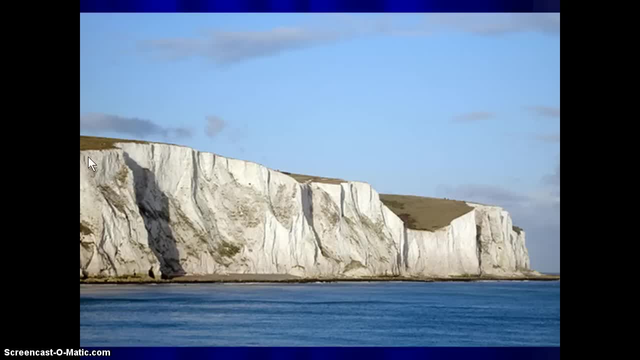 and form huge layers of biogenous sediments that eventually become rock. And here we have the white cliffs of Dover, which have eventually been uplifted and exposed from prehistoric times, And they're made up entirely of calcium carbonate, shells from microscopic organisms. 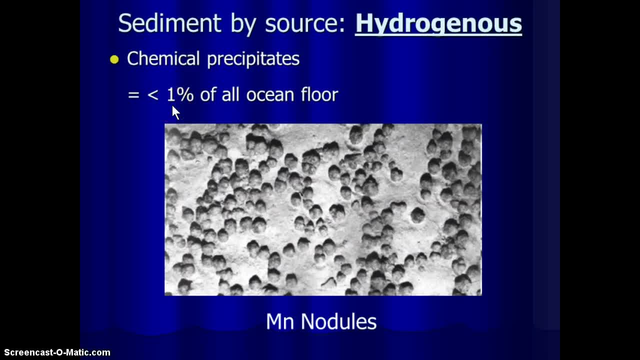 So less than 1% of the remaining sediments. So remember, the two main ones are biogenous and lithogenous, And the next biggest source is what we call hydrogenous. Hydro meaning from the water, Produced, produced from the water. I didn't write that here.